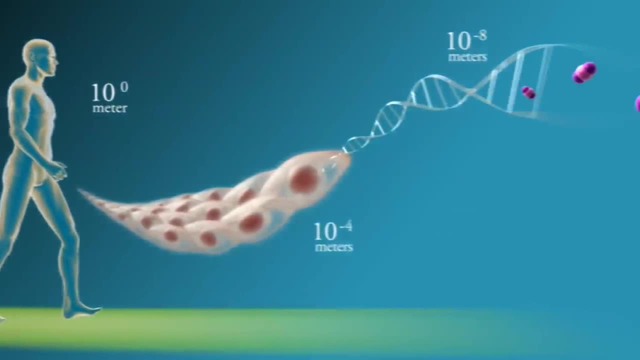 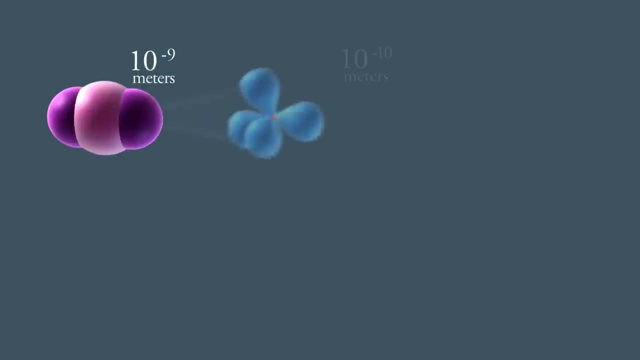 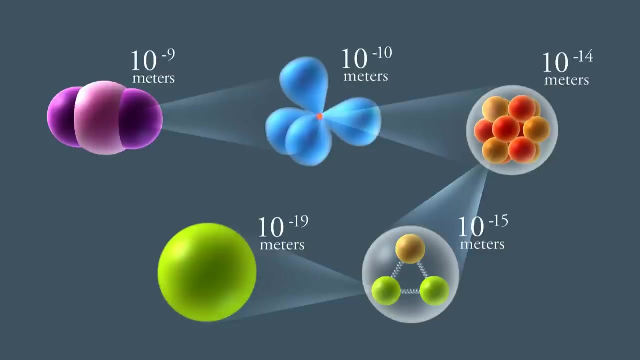 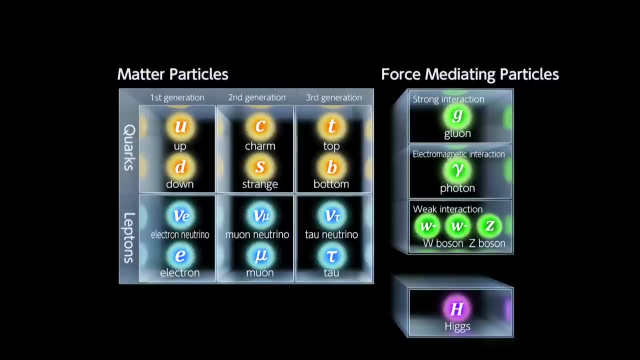 animals. nearly everything in the universe can be divided into smaller components, and Adam can be broken into a nucleus and electrons, a nucleus into protons and neutrons, which can be even further divided into quarks. these fundamental building blocks of everything in the universe are called elementary particles. recent results from particle physics suggests that the universe. 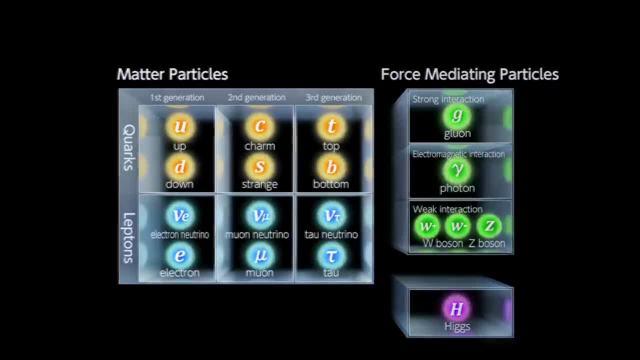 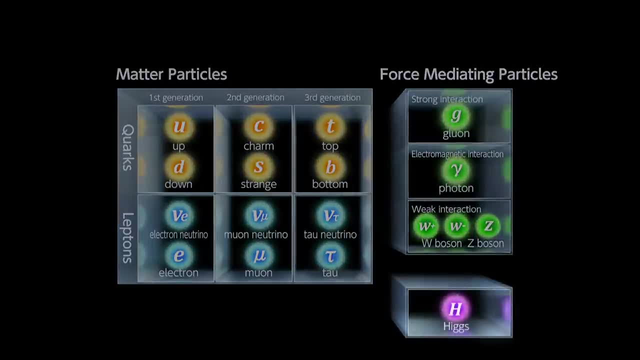 consists of the elementary particles shown in this table. quarks and leptons make up matter. bosons mediate forces between particles, and Higgs bosons are responsible for all the mass in the universe. behavior of these particles is summarized in a theory called the standard model of particle. 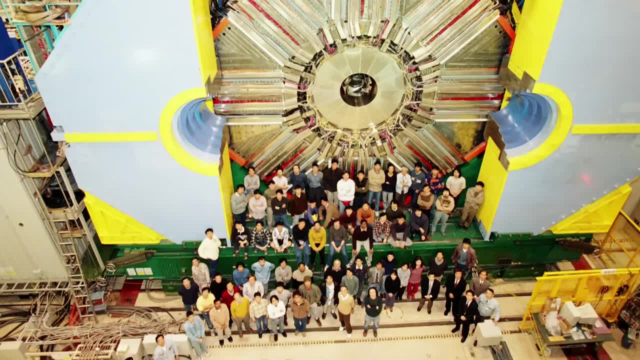 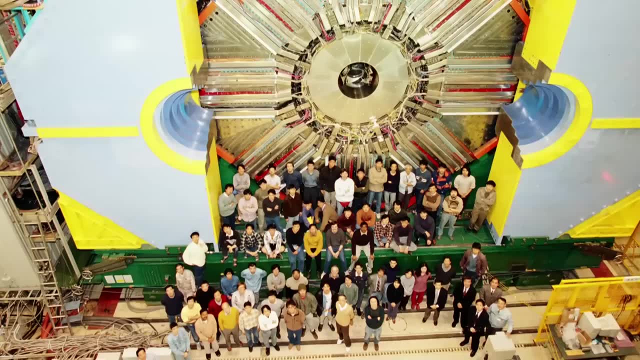 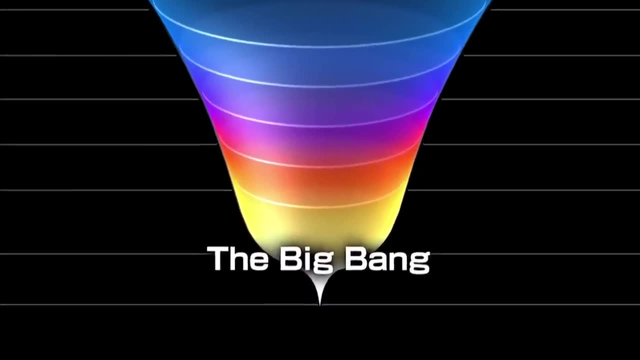 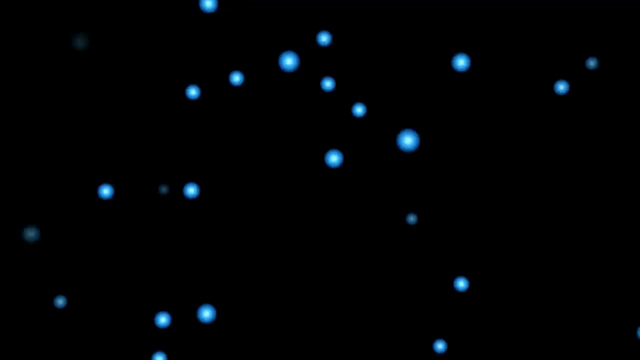 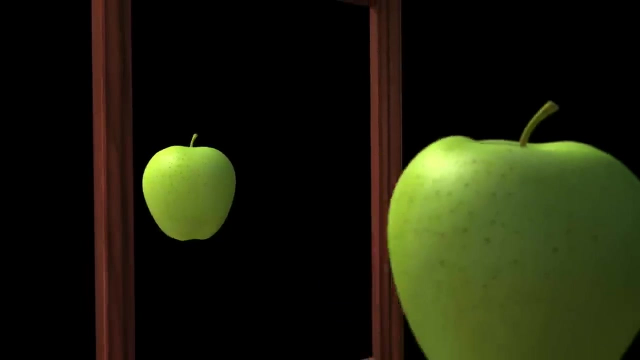 physics. the former Bell experiment produced many results that support the standard model. scientists believe that right after the Big Bang, the same number of particles and antiparticles existed. however, the universe today is only made up of ordinary matter. almost all antiparticles have somehow disappeared. for this to happen, there must be a difference in the behavior of the 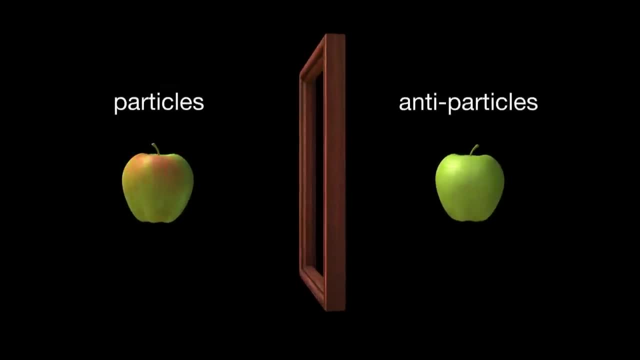 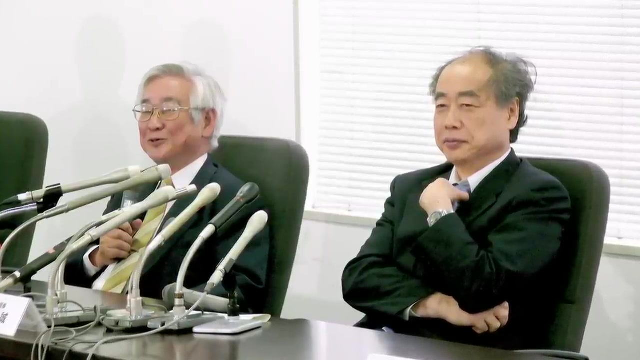 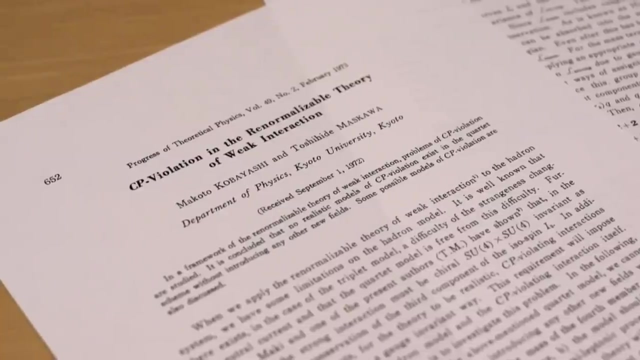 behavior of particles and antiparticles. this asymmetry in their behavior is called CP violation. in 1973, professor Makoto Kobayashi and professor Toshihide Masukawa published a model now known as the Kobayashi Masukawa theory. it was a revolutionary theory, which introduced a model that contained six quarks. even though other quarks did not have quarks, they were made up of six quarks. they were made up of six quarks. even though other quarks did not have quarks, they were made up of six quarks. they were made up of six quarks. 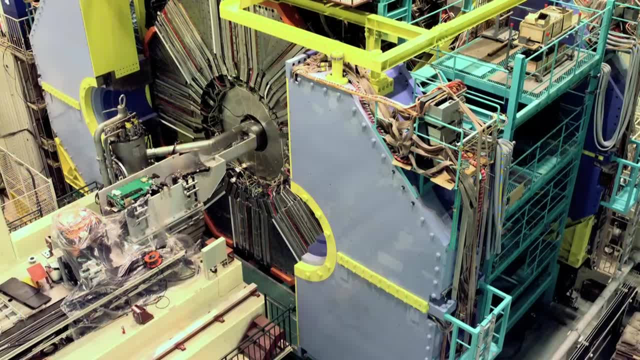 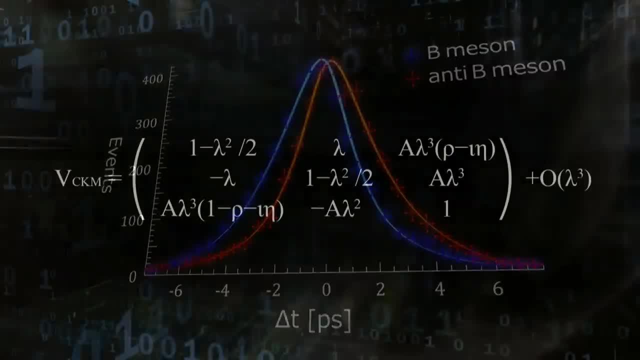 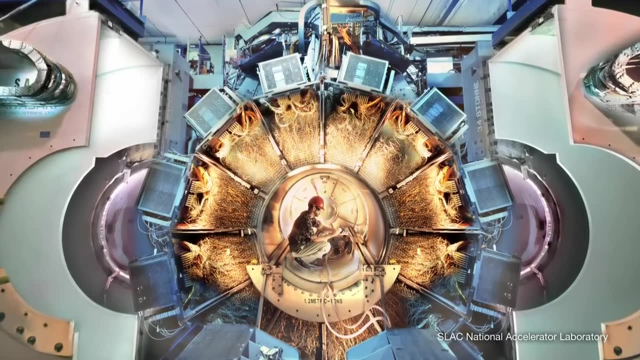 only three quarks were known at the time. in 2001, the Bell experiment successfully measured CP violation in B meson decays as predicted by the Kobayashi Masukawa theory. at the same time, the Babar experiment in the United States published a similar result in 2008, 30 years after their 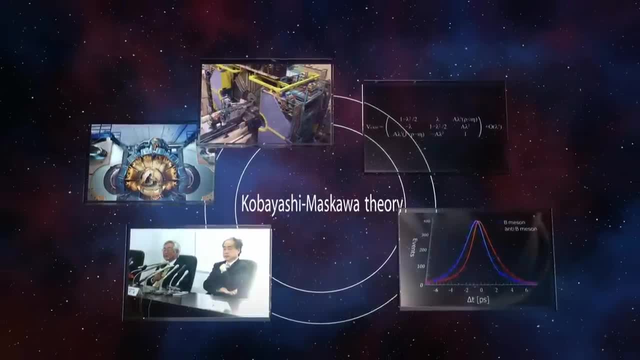 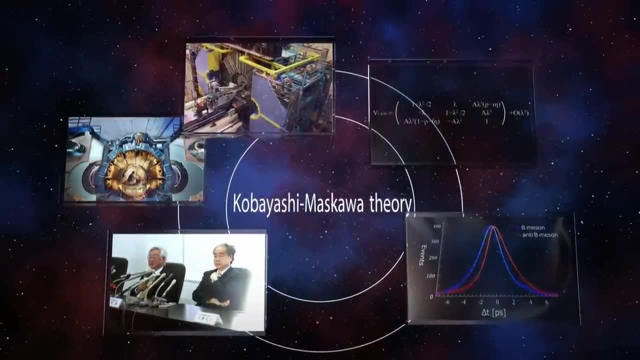 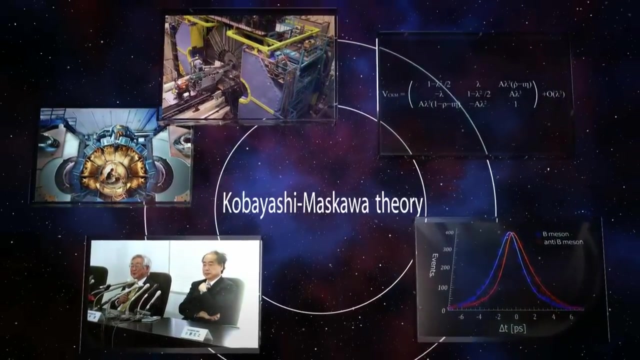 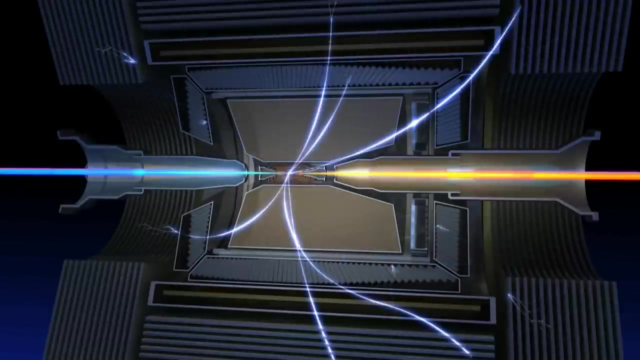 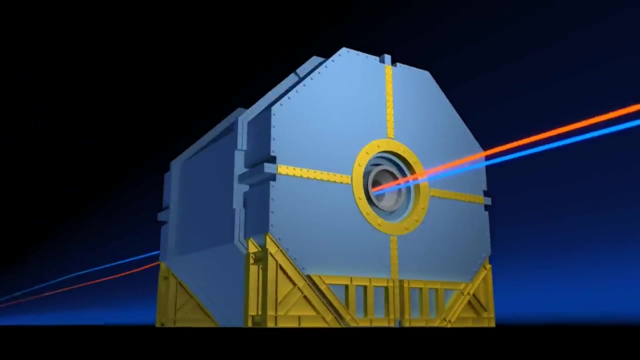 theory paper was published. professor Kobayashi and professor Masukawa won the Nobel Prize in physics. experimental confirmation of the Kobayashi- Masukawa theory by the Bell and Babar experiments greatly contributed to their Nobel Prize. let's see in detail how the bell to detector works. 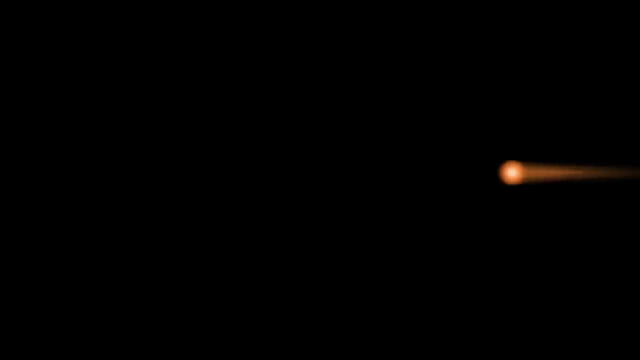 an electron and positron are accelerated to nearly the speed of light. they are then collided at the center of the B meg 이상 detector. the positron is the antimatter counterpart to the electron. when these two particles collide, they annihilate. this annihilation transforms the electron & positron. 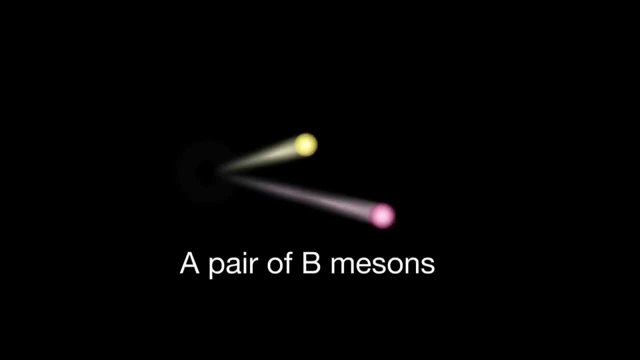 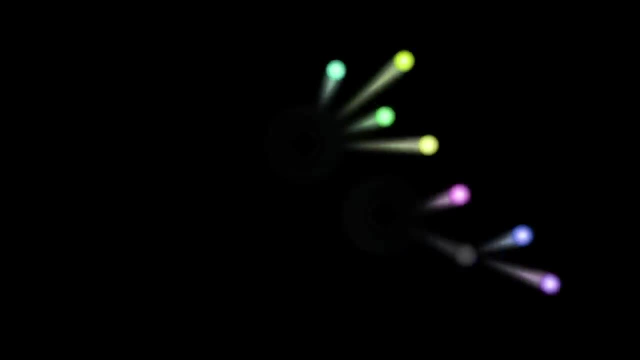 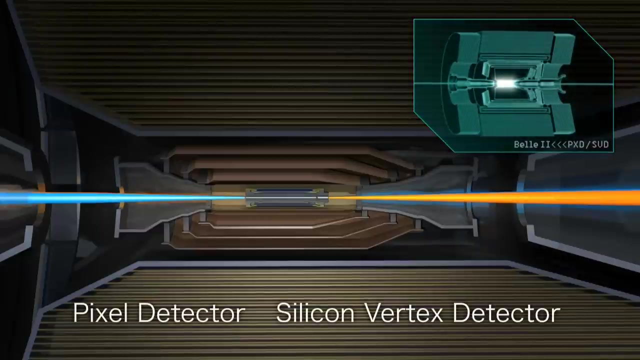 of C & V into a pair of B mesons which consist of bottom quarks. quotid想搶血? B mesons quickly decay into several lighter particles which fly away in all directions. The pixel detector and the silicon vertex detector. 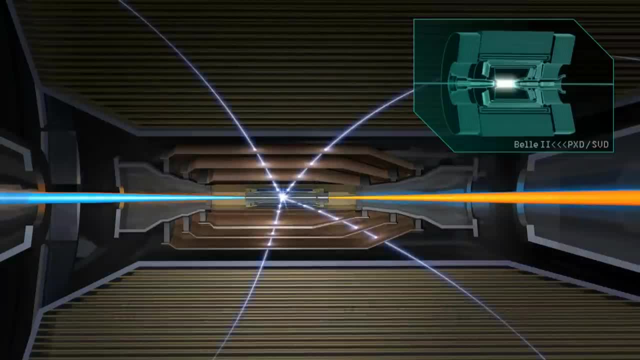 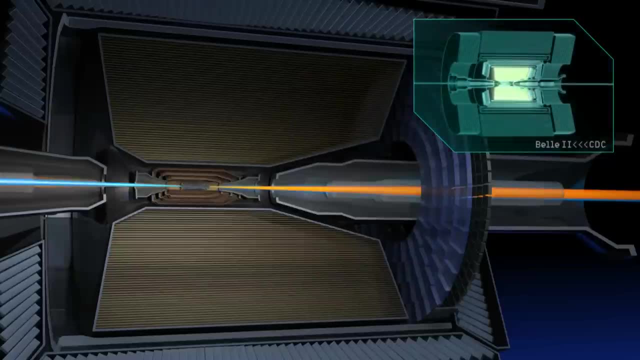 are located closest to the interaction point. They precisely detect the paths of charged particles. Particles then pass through the central drift chamber. Here they ionize the gas which fills the detector. In this way a particle's trajectory and momentum is obtained. 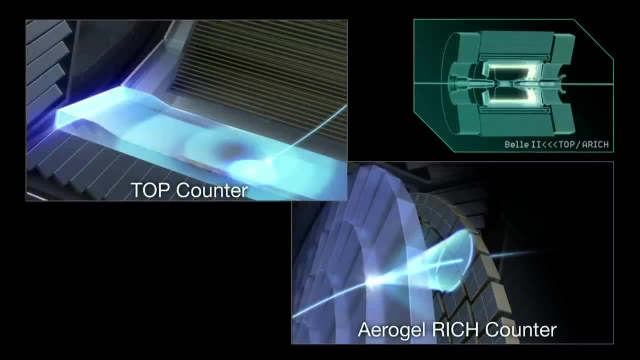 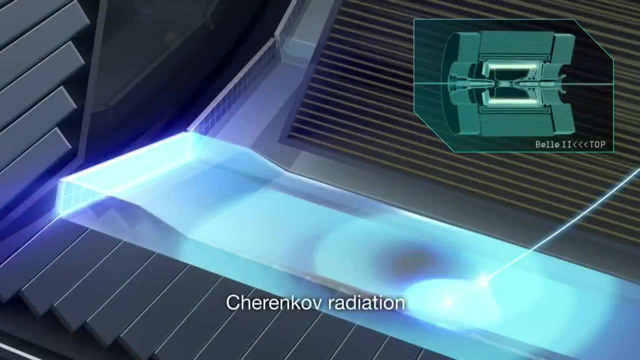 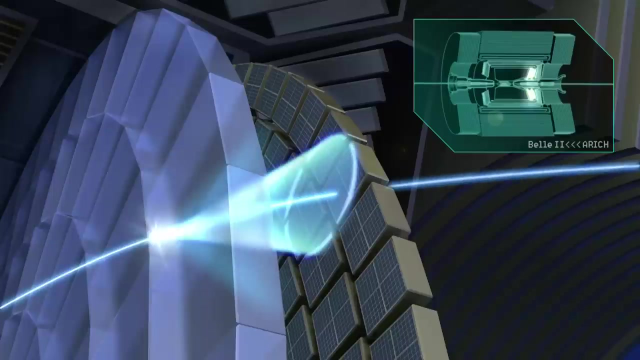 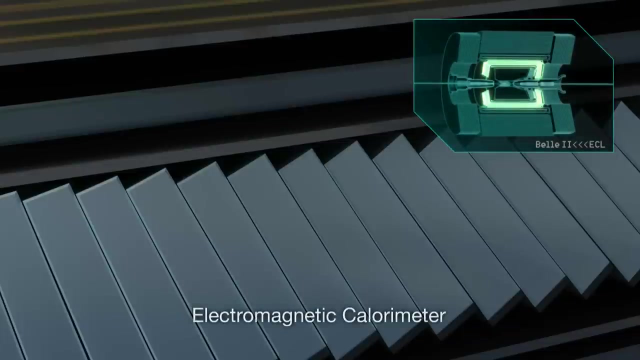 Next comes the top counter and the aerogel-rich counter. A charged particle emits Cherenkov radiation when it enters these detectors. The timing and pattern information of the detected Cherenkov radiation tells us what kind of particles it is. Then there is an electromagnetic calorimeter. 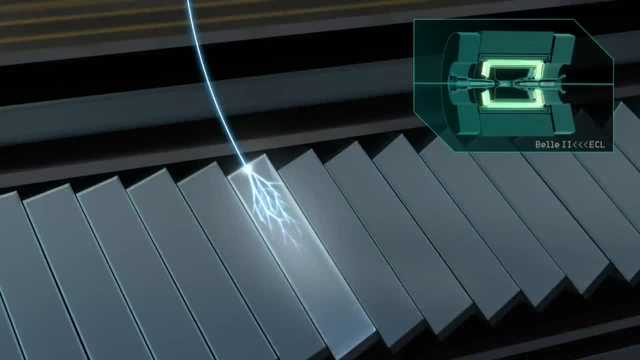 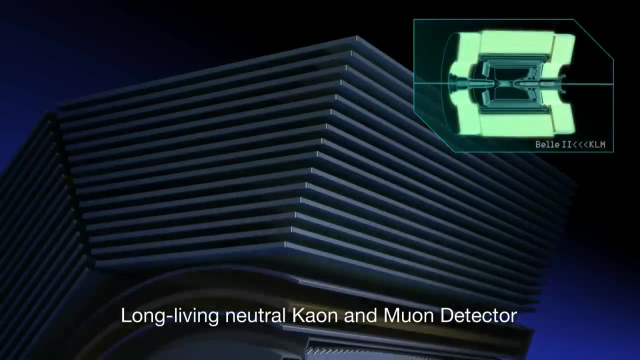 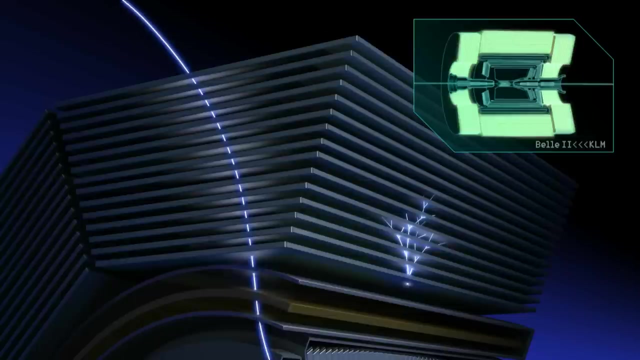 This detector precisely measures the energy of photons and electrons. The outermost detector is the long-living neutral kaon and muon detector. It detects muons which penetrate most of the detector and neutral kaons which cannot be measured with the inner detectors.